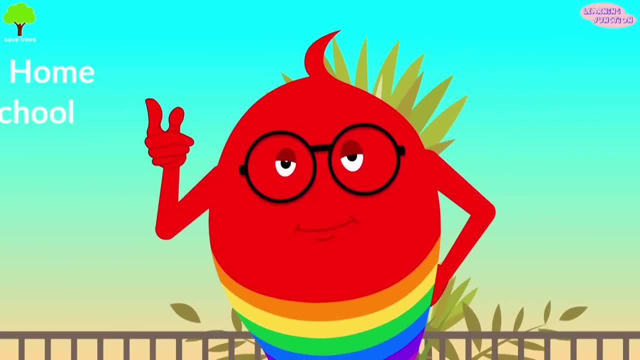 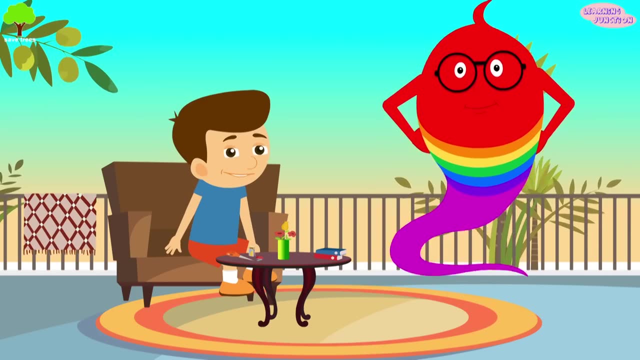 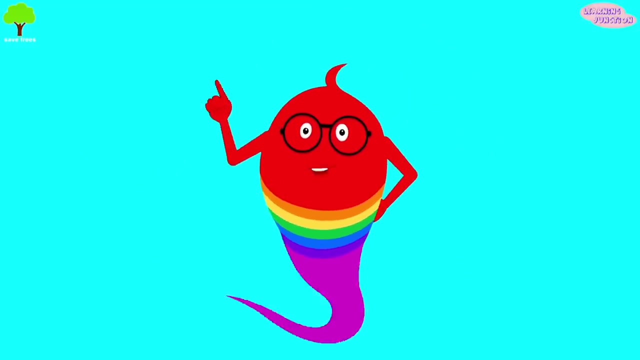 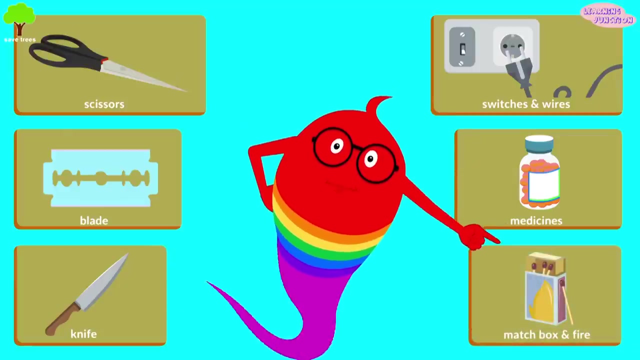 The safety rules should be followed at home, at school, on the road, and actually they should be followed everywhere. Let's learn about them today. Safety at home: We should be careful at home. Do not play with things like scissors, blades, knives, switches and wires, medicines, matchsticks or fire. 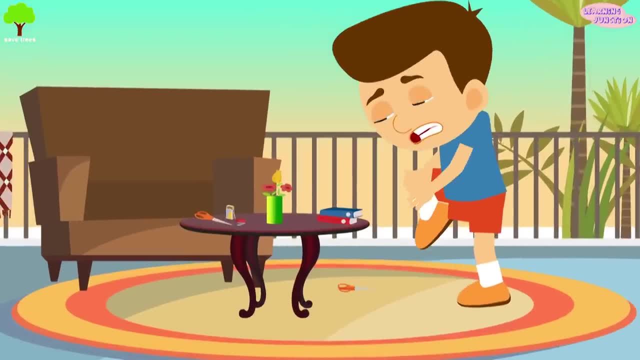 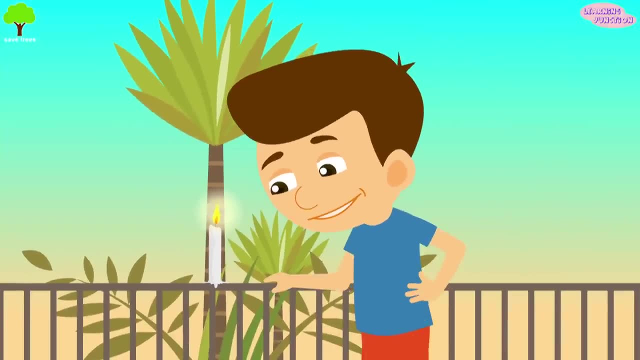 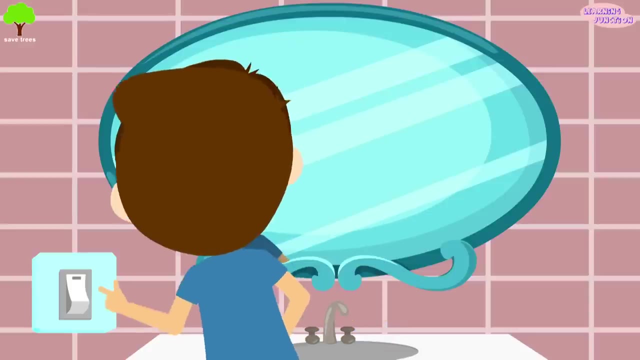 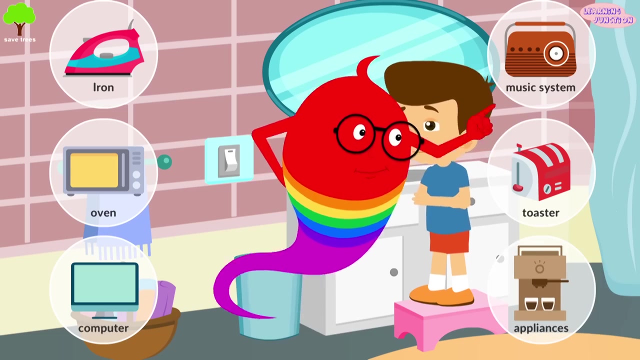 These can be extremely harmful for us. For example, if you play with scissors you might get cut, And playing with fire is dangerous. You may burn yourself or your house may even catch fire. Do not touch electrical equipment like switches and wires, hot irons, the oven, computers, music players, toasters and other electrical items with wet hands. It may give you an electric shock. 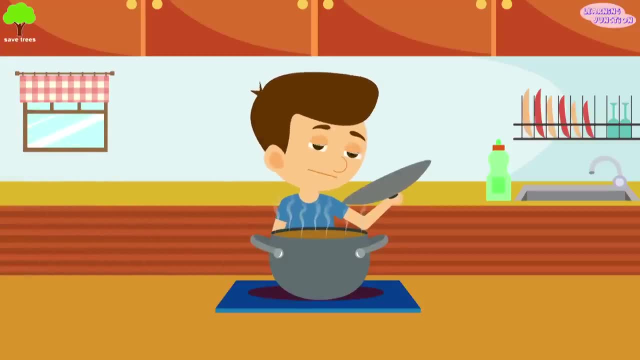 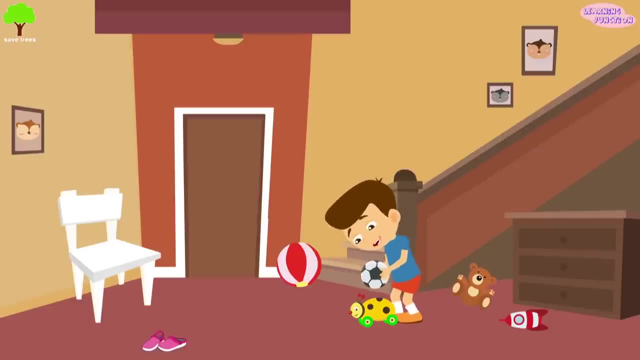 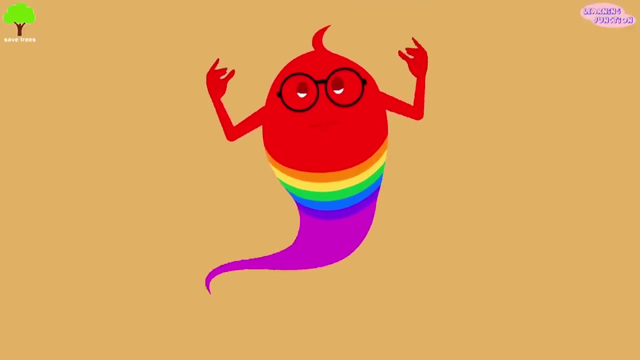 Do not go near the stove or touch the hot pans in the kitchen. Keep your toys, bags, shoes and other items in place. You or anyone else could fall over them. Be careful: Never open the door for strangers. They may harm you. 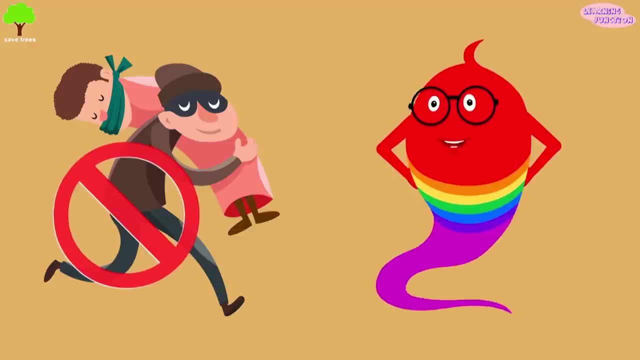 While most people are good, there are some people who are not and do not keep kids safe. Don't be tempted by people you don't know. Now we'll learn some safety tips for school and school lessons. Now we'll learn some safety tips for school and school lessons. 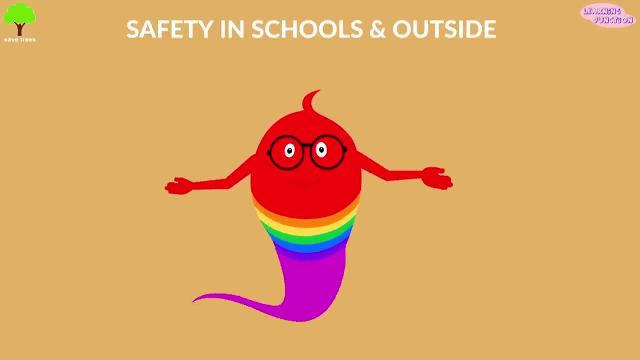 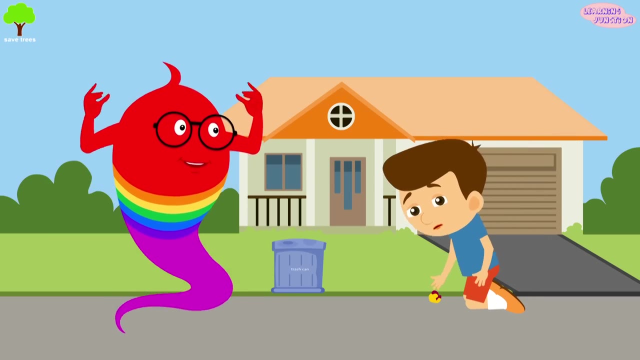 Now we'll learn some safety tips for school and school lessons. tips for school and outside: Ah, always throw the waste in the dustbin. buddy Littering by throwing waste here and there pollutes the land and makes it unsafe. 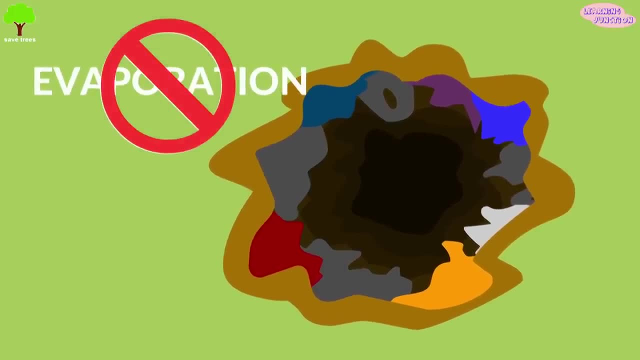 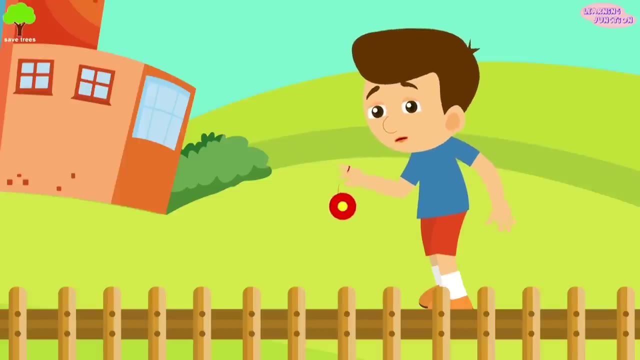 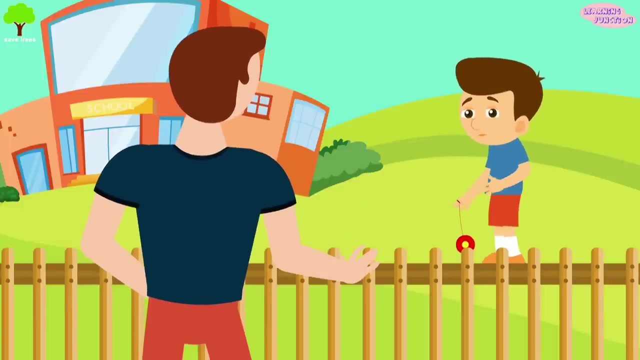 It poses a big health threat to animals and humans. We should always walk in a queue, Wait for your turn and do not push anyone. Do not ever leave your school or go anywhere with a stranger. Do not eat anything given to you by a stranger. 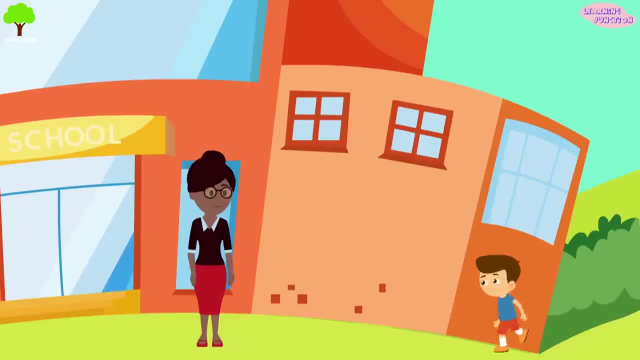 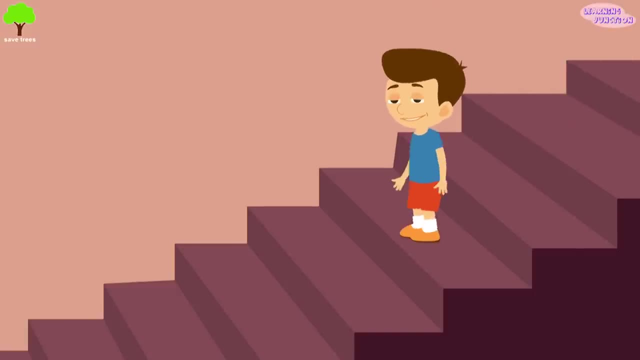 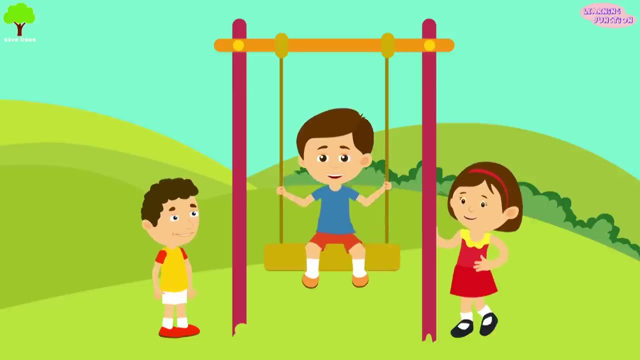 It may be harmful for you. Remember to inform your teacher or school security if you see someone suspicious. Be careful on stairs. Do not push anyone or run and jump on the stairs. You may hurt yourself or others. When you're on the playground, always wait for your turn on the swings.